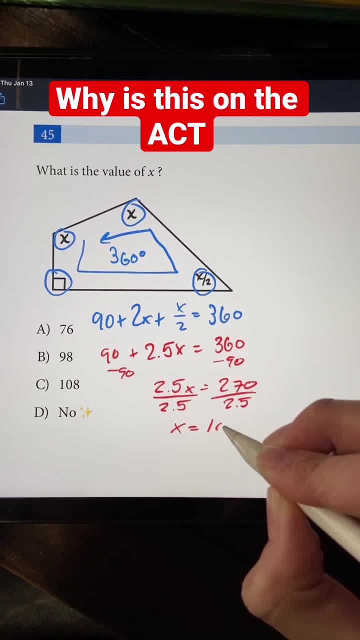 2.5 to get x. by itself- and we're going to get x- is equal to 108, which is choice C.